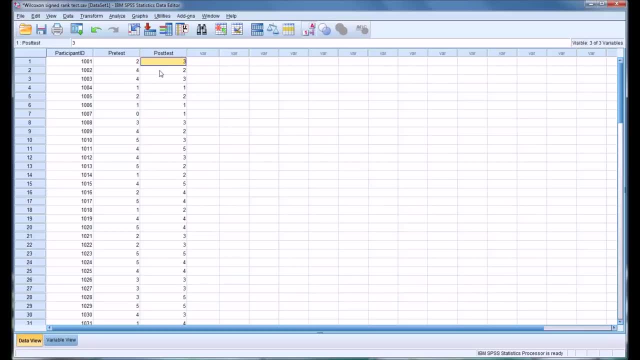 of depressive symptoms It will reduce as well. In this test that will be realized that the average of depressive symptoms that we have is probably eight. So we're measuring the severity of dep stimulating symptoms And the scoring will be four And this symbol. 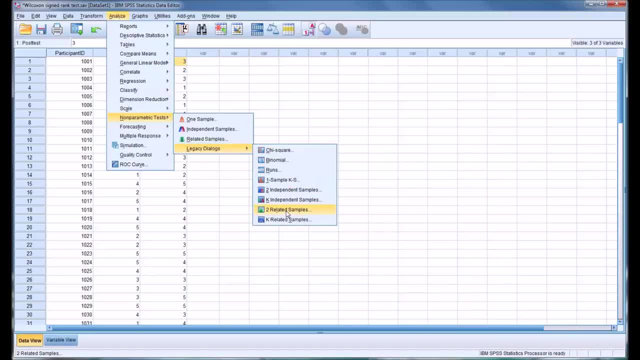 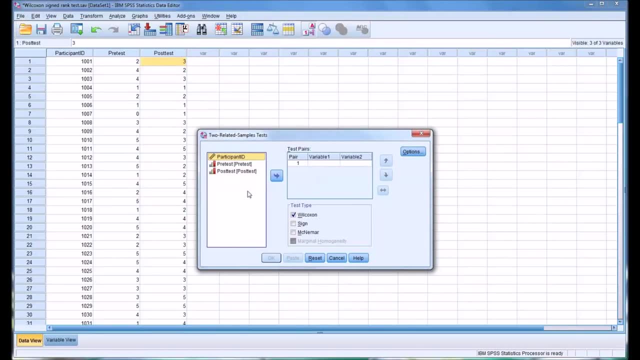 in�� of these is the dev siege crimes. In this sample count of dep pipe depends on the From this dialog to Related Samples Test. I'm going to put the pre-test in Variable 1 and the post-test in Variable 2.. Wilcoxon is checked off by default as the test type and the options I'm going to leave the same, except for I'm going to select Descriptive Statistics. 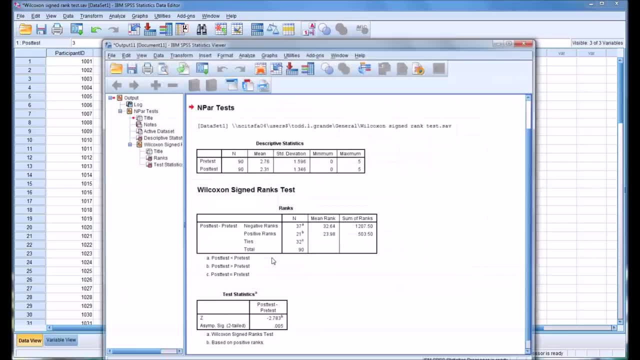 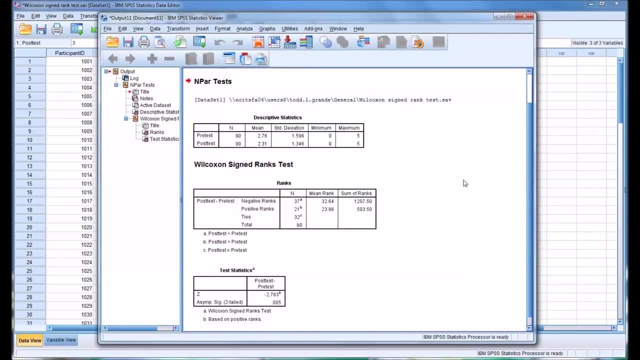 Click Continue, then click OK And you can see the results are fairly straightforward. There's three tables. In the first table you can see that there's 90 pre-test scores and 90 post-test scores. Both variables had a minimum score of 0 and a maximum score of 5.. 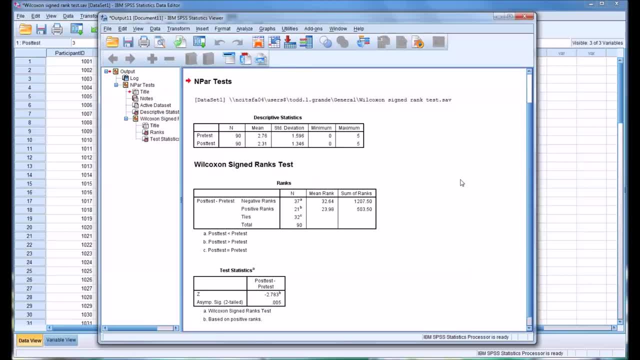 The standard deviations are provided And you can see the mean for the pre-test is higher than the mean for the post-test. So before we even look further down at the other tables, we know that it's looking good for our hope that the post-test would be lower. 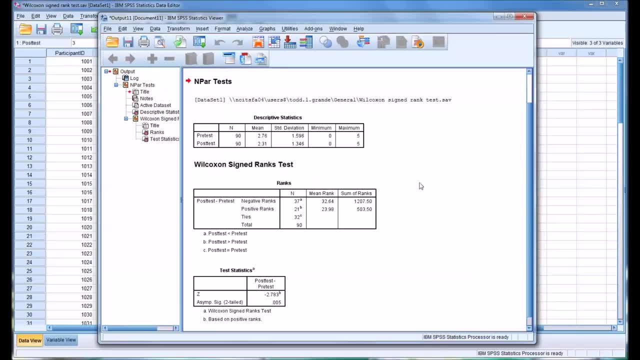 Without looking down further, we wouldn't know if there's statistical significance, But we know the direction, and that is that the post-test is lower. The mean is 2.31 for the post-test and 2.76 for the pre-test. 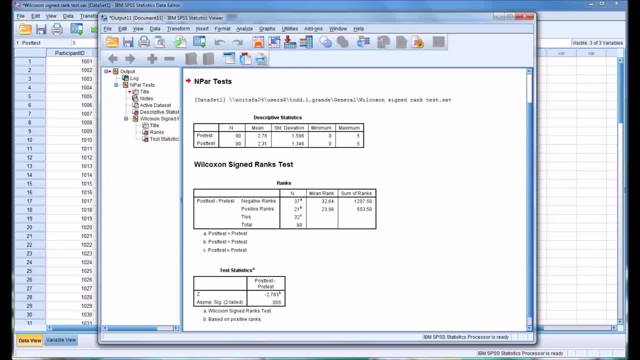 So then, moving down to the ranks, SPSS provides us the number of participants that have negative ranks, positive ranks and ties. So what that means in this case is that there were 37 cases where the post-test score was lower than the pre-test score. 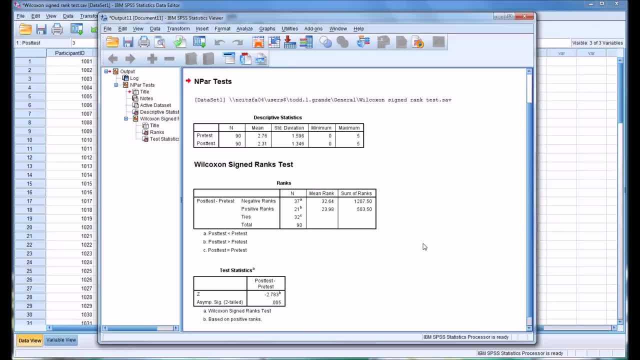 which is, of course, what we want. That's what we'd be hoping for. There were 21 cases where the post-test score was higher than the pre-test score, So in that case, the participant had a higher severity of depressive symptoms as measured on the post-test. 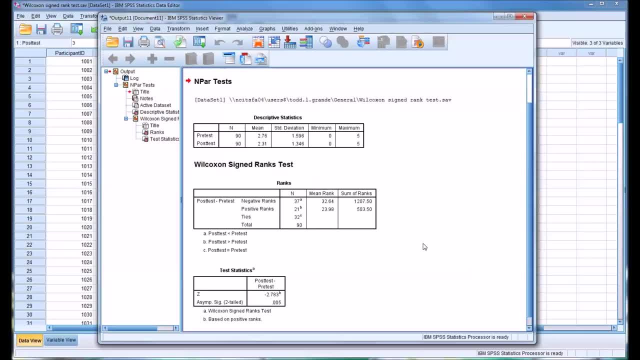 And then there were 32 cases where there was a tie, That is, the post-test was equal to the pre-test. So as we look down at the test statistics, we see the Z is negative 2.783, and the significance is 0.005.. 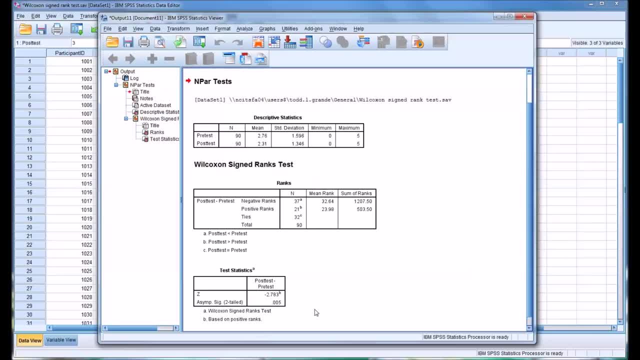 So if we set the alpha at 0.05, which is fairly common in the social sciences, this would be statistically significant. So we would reject null hypothesis. We would presume there is a difference here between the pre-test and the post-test. 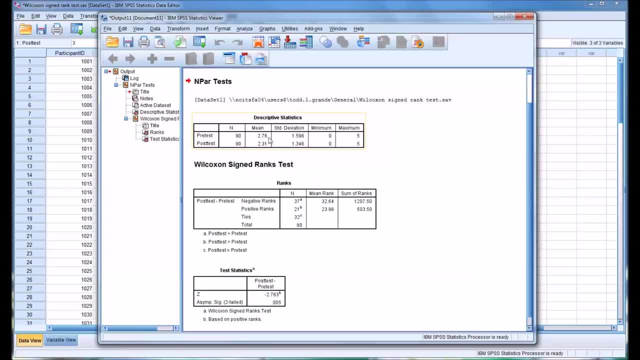 And we know from this descriptive statistics table that the post-test was lower. So the direction of the difference is that the severity of symptoms decreased as measured by the post-test when compared to as measured by the pre-test. So in analyzing this data we would presume that the treatment was successful. 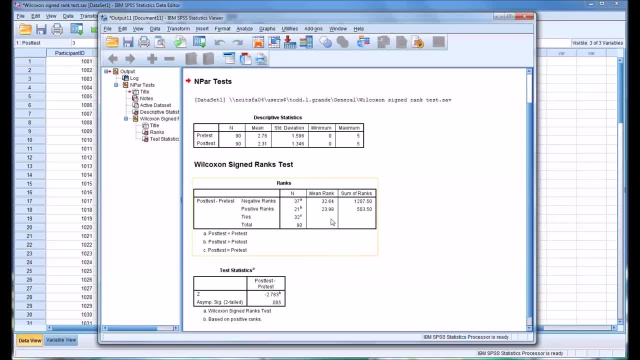 So it's important to note here that if you look at these ranks a little more carefully, there's 21 instances here, 21 cases, where the post-test score was greater than the pre-test, So we would hope, of course, the post-test would be lower. 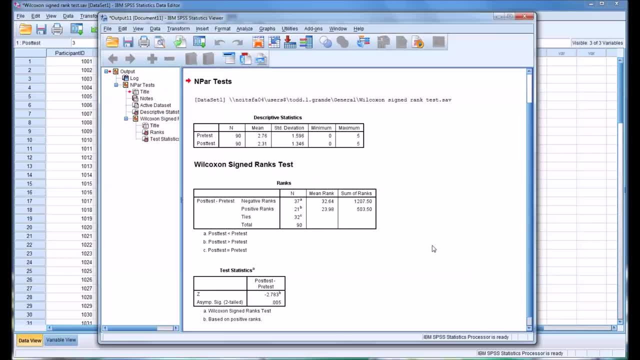 So there's 21 instances where the severity of symptoms were higher, and then, of course, 32 where there was no change. So there was only 37 out of 90 that actually improved. Another important aspect to look at is the sum of the ranks. 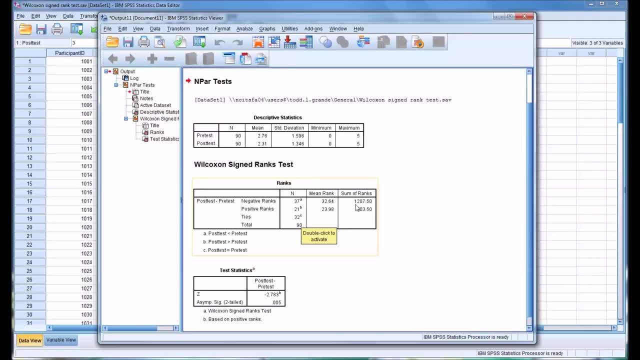 which is also provided here as 1207.5 for the negative ranks and only 503.5 for the positive ranks. I hope you found this video on the Wilcoxon sign rank test to be useful. As always, if you have any questions or concerns, feel free to contact me. and I'll be happy to assist you.